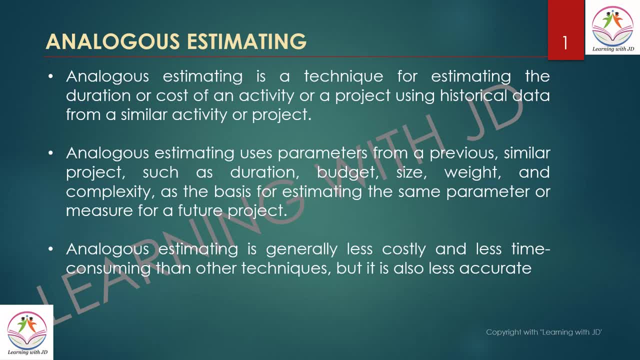 you are working on a project, um, you know, you have shorter duration of time for planning. sometimes it happens that you have shorter duration of plan for time for planning and in that case your manager may just come back to you and say that you know, hey, uh, we want to plan for an activity or for a 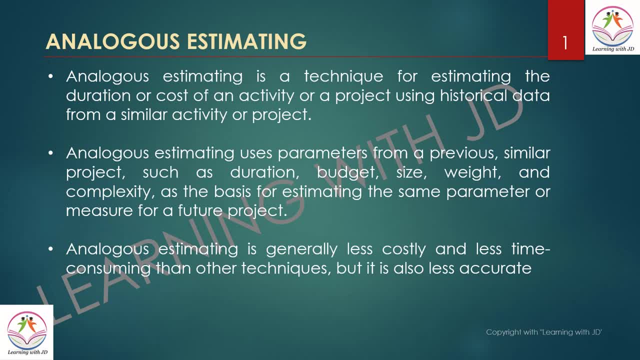 project. tell me, what do you think? how long will it take in that case? what you do generally is you try and see that if something, some project or some activity like is there, is a part of your historical information, and if you get that information you try and analyze on the same. 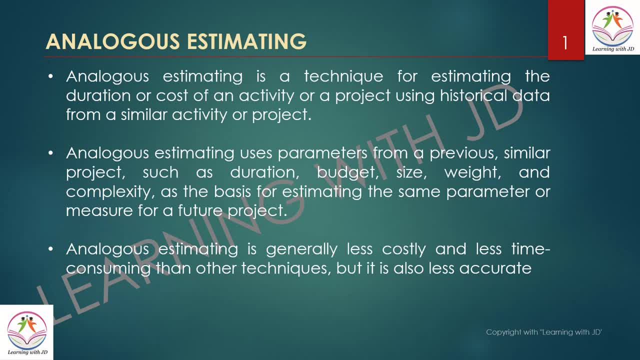 basis, which means analogous estimating, is a technique for estimating the duration or cost of an activity or a project using historical data from a similar activity or project. if such activity is done, then you can try and see that if something is, there is a part of your historical. 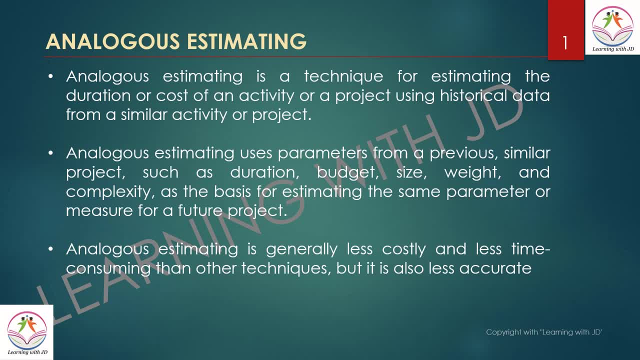 information and if it has happened previously and if it has taken, say, seven days, you will say plus or minus. uh, you know, nine days or five days is something that your activity will take. analogous estimating uses parameters from the previous similar project- not like a different project, but a similar project- such as the duration, the budget, the size, uh complexity, the weight. 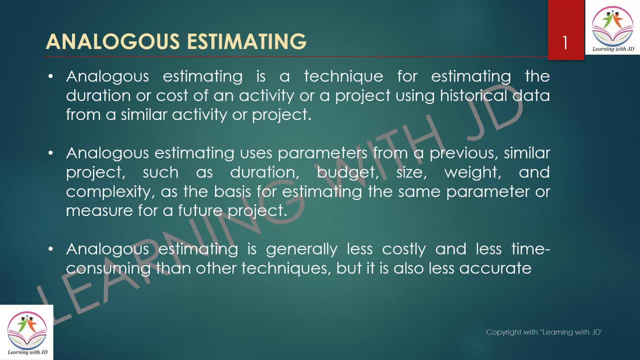 right as the basis for estimating the same parameter or measure. you can try and see that if something is there is a part of your historical information and, if so, for a future project- the project that you're working on- you can take your background from the similar previous project. analogous estimation is generally less costly because you've not put 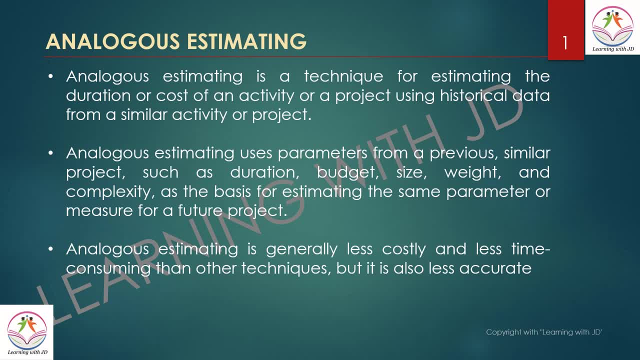 lot of time and effort in that and less time consuming because the data is available to you. it's quickly available than any other technique, but it is also less accurate. understand that you have not done too much research on it. right, you have just taken the information from the. 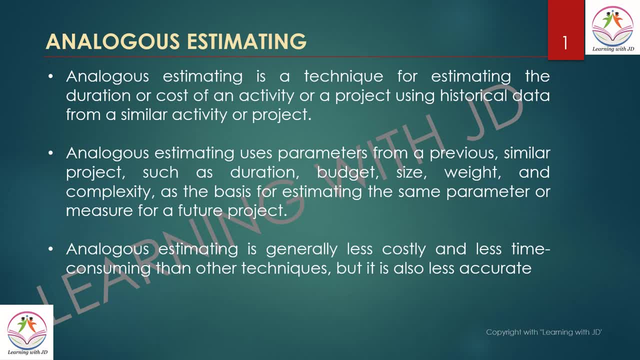 previous project, and while you're informing this to the sponsor, to your manager, to any stakeholder that you know, this time, uh, this activity will take so much time or will have need so much cost, what you need to do is that you also need to tell them that i'm using the method of analogous. 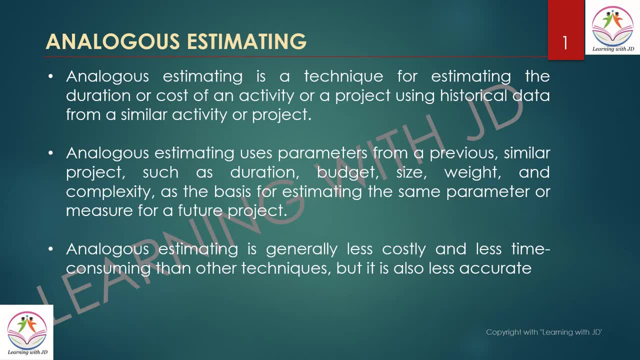 estimating. now, how does this impact you from your examination perspective? you may get a question saying that you are working on a project, but you don't have too much time. uh, you search or you dig on the lessons learned and you find out that a project was already done on the similar lines and 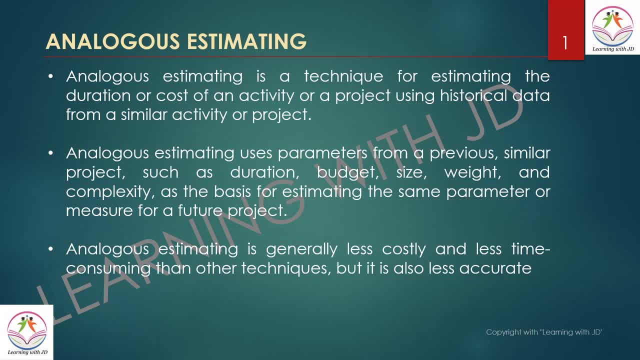 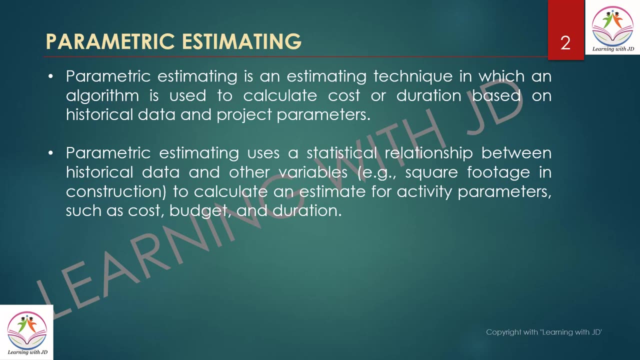 it's on similar kind. uh, what kind of estimating technique do you think suits best? so it will be analogous estimation. got that, let's see the second one, parametric estimation. now there's a very thin line between analogous and parametric estimation. parametric estimation also takes the data from the. 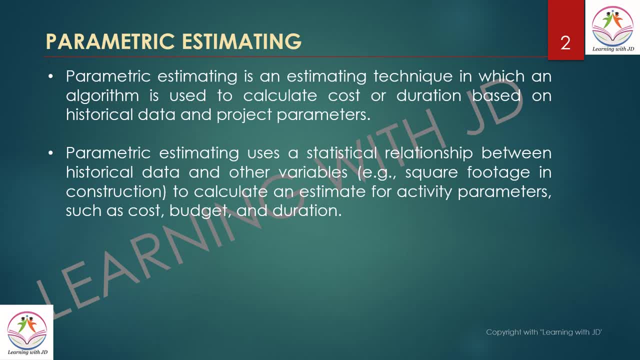 historical data and project parameters. additional thing which is added as a part of the parametric uh estimation is that it also takes some value from the previous project, for example, that uh for calculating the cost. uh, it has taken, uh, say, 10 rupees per square feet will be the cost was the. 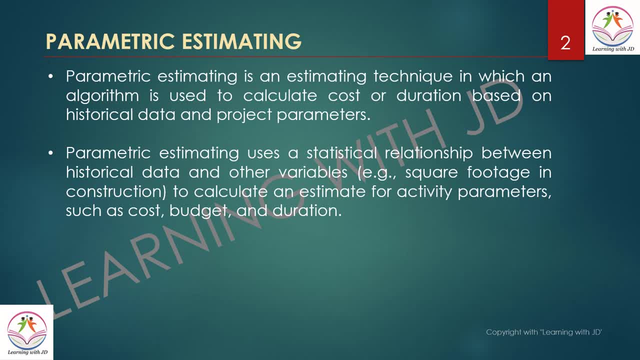 cost of the previous project or at that point of time, uh, the labor had charged 500 rupees per day. so the moment you add some statistical relationship between the historical data and other variables, for example square footage and construction or any other, to calculate and estimate for the activity parameters such as cost, budget or duration, it is a parametric. 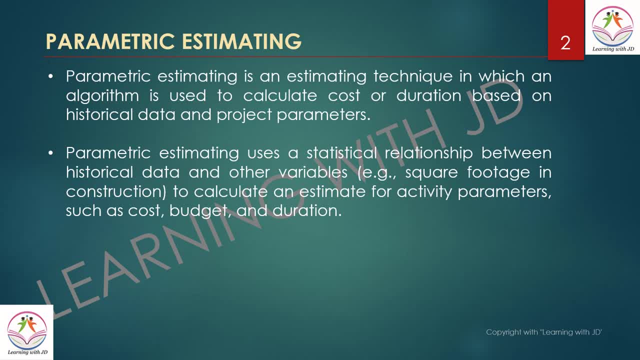 estimation. so understand, uh, that when you get an exam question and it is mentioned that you know um, you have seen that in the previous project 10 rupees per square feet was was used in construction, and that's in statistical information which is available. what kind of 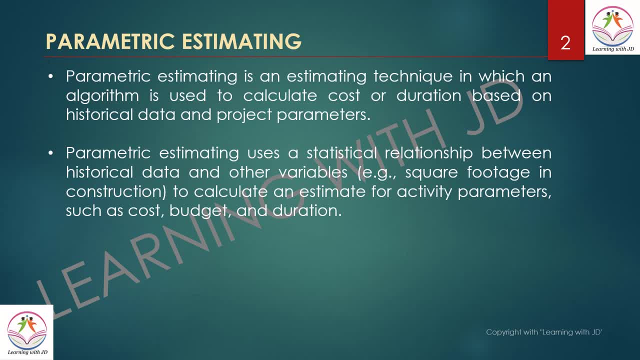 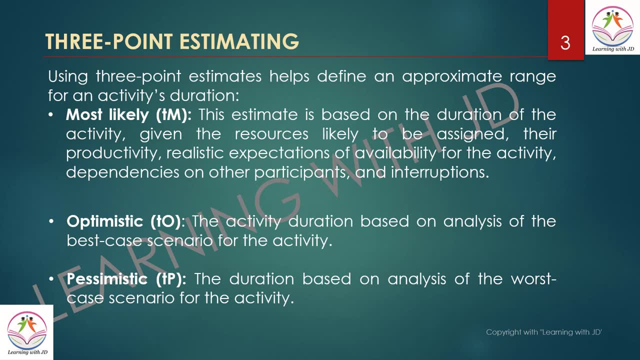 estimating technique are you using? it is a parametric estimation. now comes the three-point estimation. so using a three-point estimation that helps define an approximate range for an activities duration. now you will definitely get one or two mark. question on three-point estimation. it's a simple calculation. you need to remember this and you will easily crack one or two marks. 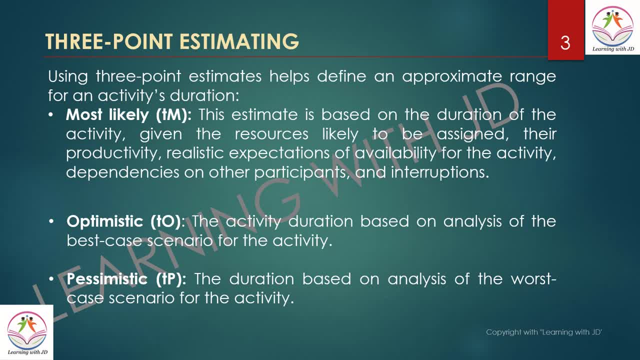 here, so do not mess out here. okay, so there are three parameters that will be given to you, okay, one is the most likely. two is the optimist figure. three is the pessimist figure. so let's take an example, for example, that there is an activity that needs to be completed. you feel that in the 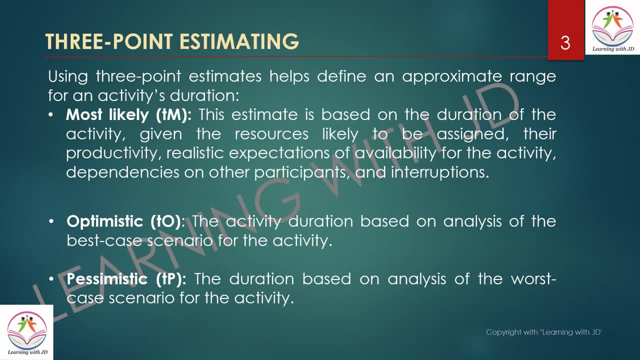 most optimist scenario, you will be able to finish this activity, say, in five days. the most pessimistic scenario is, say, 15 days, and most likely say 12 days is what you will finish this activity in now. this is the kind of estimation that needs to be done and there is a formula around this that 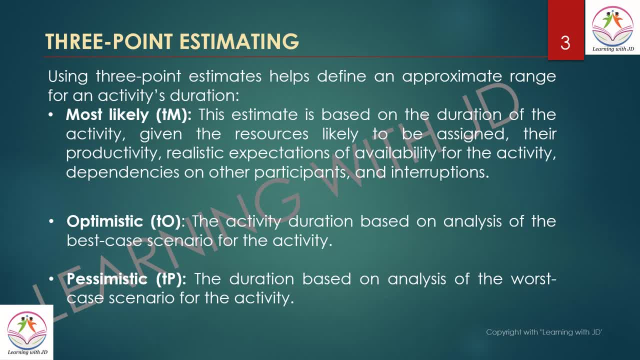 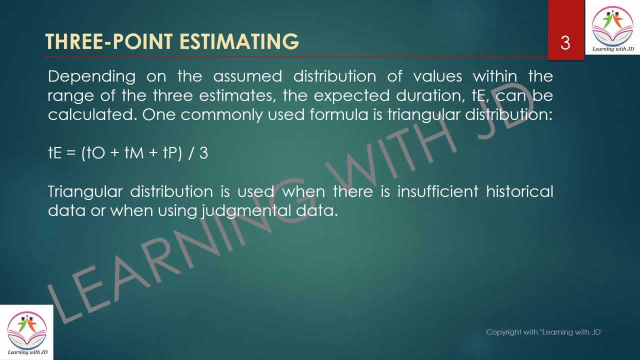 as to how will you find out the three-point estimating value, which is t e. so t e is assuming we are taking time into consideration here. if it is cost, it will be c e, so t e is time t o o plus m plus p, which is o, is the optimist figure. so our optimist figure here was five. most likely was uh 12, so 5. 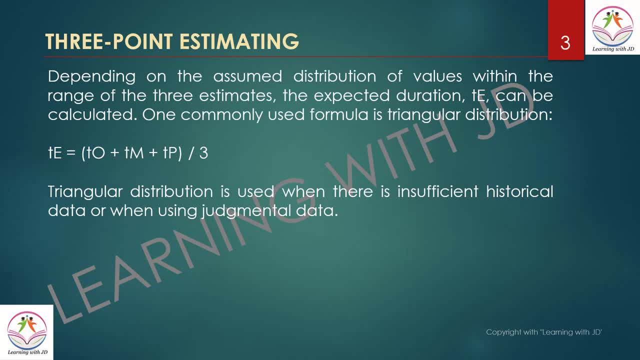 plus 12 and plus p, which was the most pessimist figure, which was 15. so which is, uh, 5 plus 12 plus 15 is equal to 32, and you need to divide 32 by 3, which is 10.66, right? so which means that, as per, 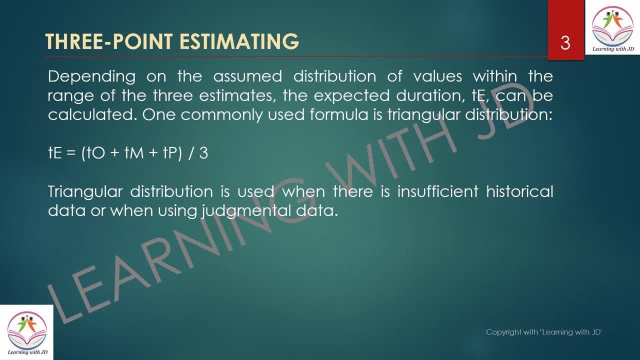 estimation, you will be able to finish this particular activity in 10 days and say, a few hours right, 10.66. okay, so that's the way you find out the three-point estimation. have you got it? see, guys, this is really important from your examination perspective. just understand that. 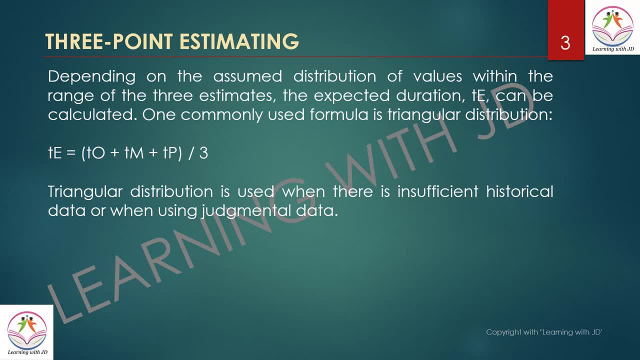 these three values of o, m and p, which is optimist, most likely and pessimist- will be given to you from your examination perspective. you just need to use the formula and get to a number right and if it does, you will get the correct answer. that can. 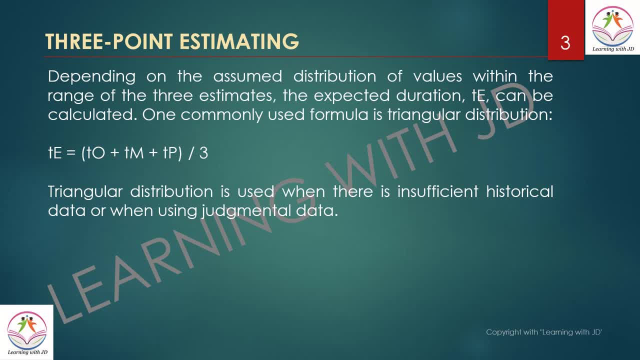 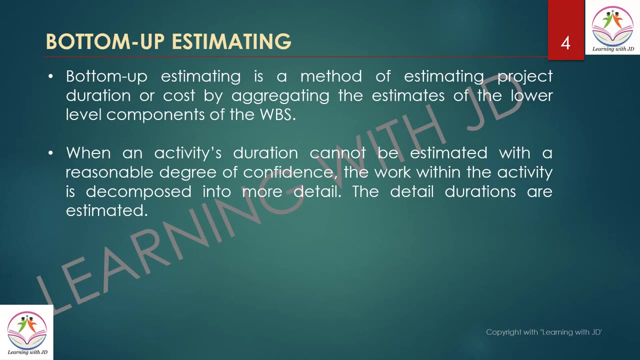 be one kind of question. and the second kind of question is that you are calculating by taking a mean or you're calculating by taking three scenarios. what kind of estimation are you using? it's a three-point estimating technique. got that. so these three are the most key ones and the last. 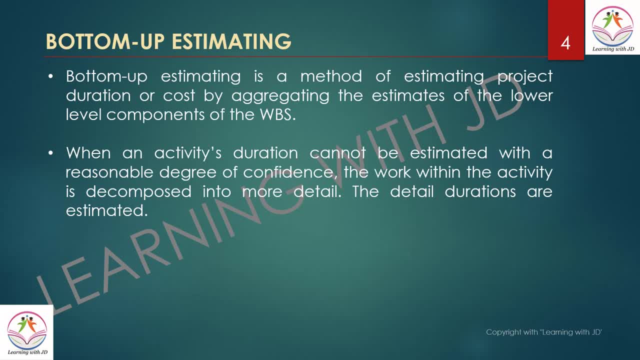 one is the bottom-up estimation. so bottom-up estimation is the method which is estimated as the planning of the project progresses, for example, and it is more accurate as well, which means that you plan the project activities at the lowest level, say at the WBS level, right at. 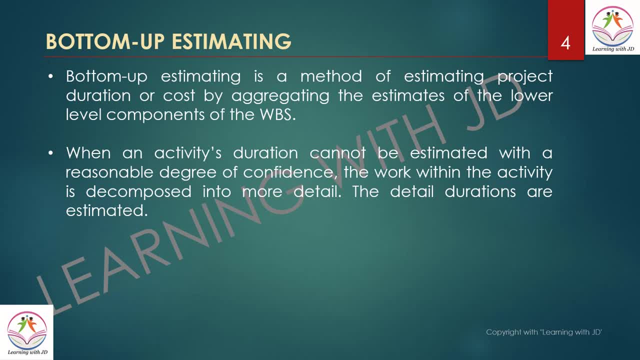 the work breakdown, structure level, and then you aggregate it to come up to an estimate. so for each activity you will know that this activity will take two days, three days, one day, whatever, and then you add all that and then you come up with a very, very approximately accurate project timeline. 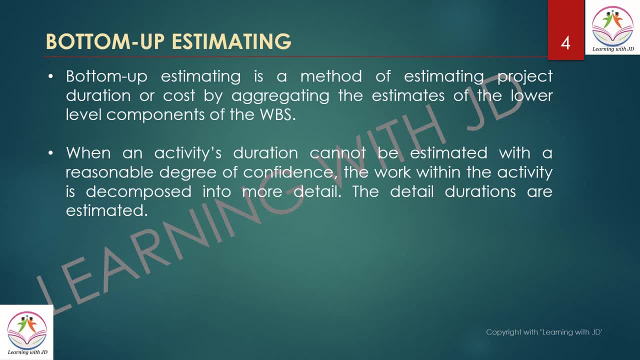 which will say that, okay, you will finish this project in this particular timeline, and that's what is known as bottom-up estimation. so let's see what it is. bottom-up estimating is a method of estimating project duration or cost by aggregating, right, I told you, you aggregate. 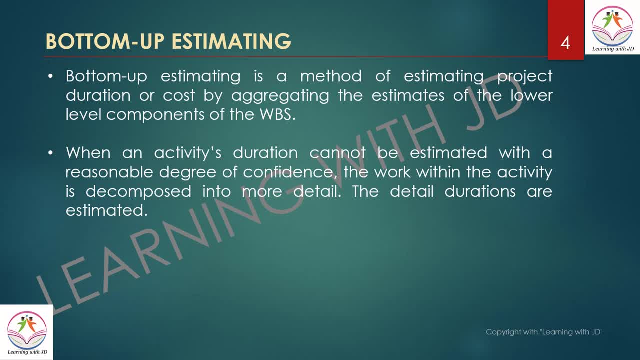 the estimate of the lower level component of the WBS. when an activity's duration cannot be estimated without a reasonable degree of confidence, the work within the activity is decomposed into more detail. so if there is an activity that you're not able to estimate, you further break. 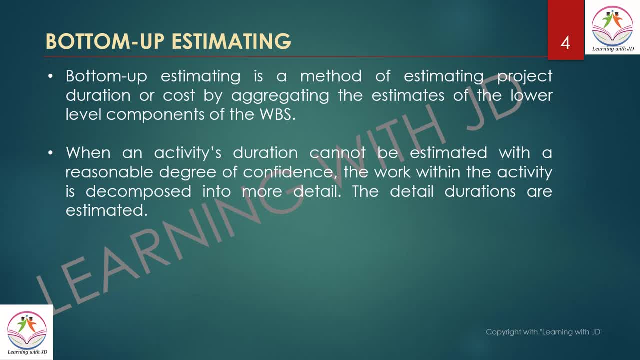 it down, you further decompose it at the level where you can estimate it. the detailed durations are then estimated. so these durations- whatever you you know, these activities, whatever you break down or decompose, are further estimated. you roll it up and you create your bottoms-up estimation. 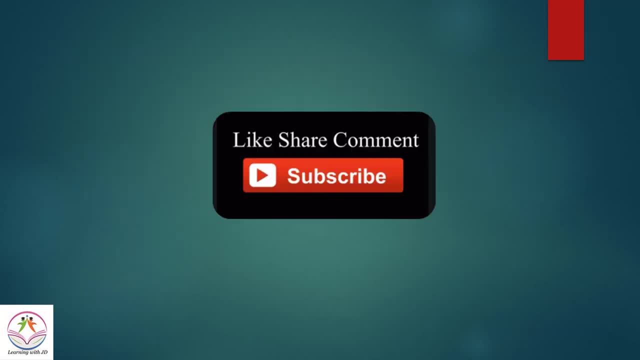 so guys remember analogous estimation, parametric estimation, three-point estimation and bottom-up estimation. analogous is less costly, less time-consuming and also less accurate. parametric also less costly, less time-consuming and a little more accurate than analogous. be why: because you have some statistical relationship with the historical data. third is three-point estimate. remember O plus M plus P. 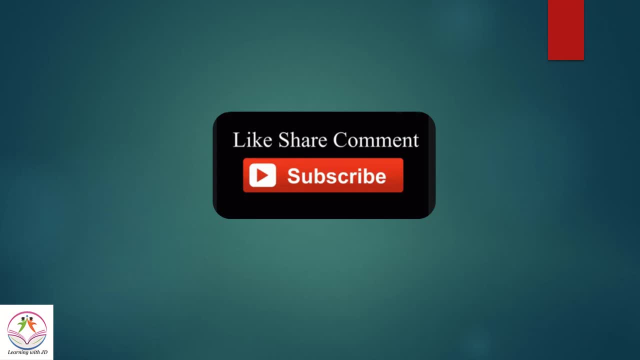 divided by three, and the fourth one is bottom-up estimation, which is the most accurate but time-consuming and also costly. I hope this topic is clear to you. thank you for hearing me out. or do like share and comment on my video and I will definitely come back to you. if you have any queries, do do subscribe to my